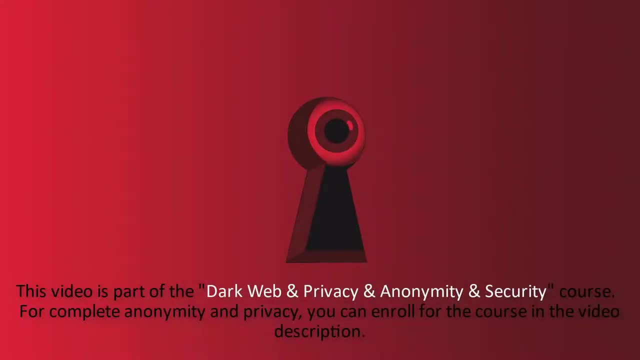 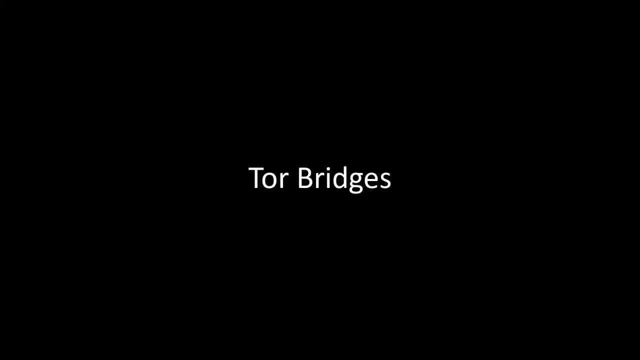 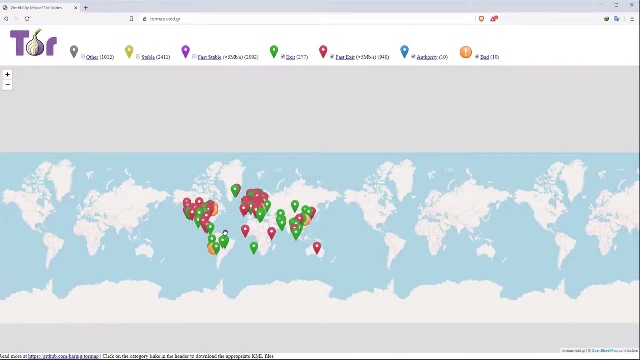 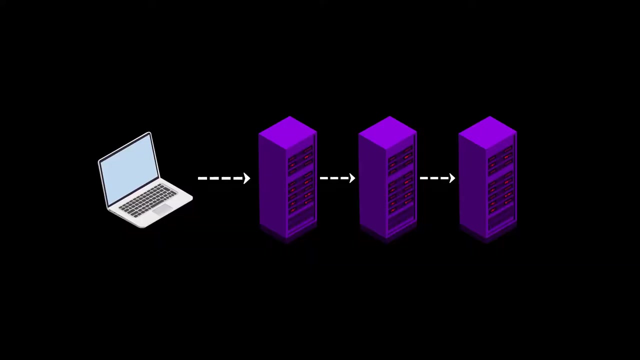 When I talk about the working structure of the Tor network. at the beginning of the course I mentioned that the list of the server in the Tor network is publicly published and therefore the Tor servers can be easily blocked. Authorities, such a government, your service provider or your network administrator can easily blocking the Tor network through this. 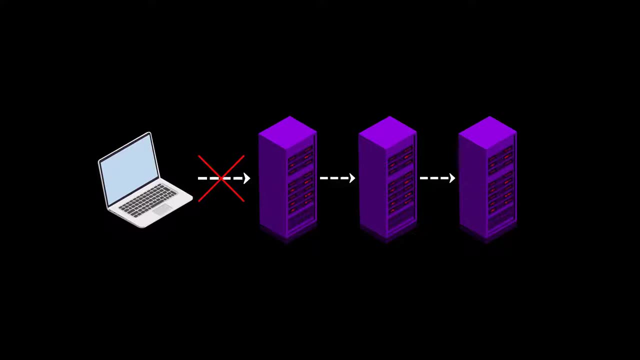 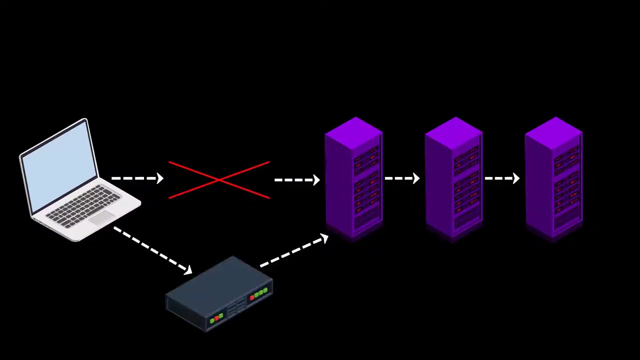 publicly published the list of servers. It's possible that you will often encounter situation where the Tor network is blocked, because it is easy to block. In such a cases, you can use the bridge connections provided by Tor project to overcome the obstacle, Since the list of bridge routers is keep confidential. 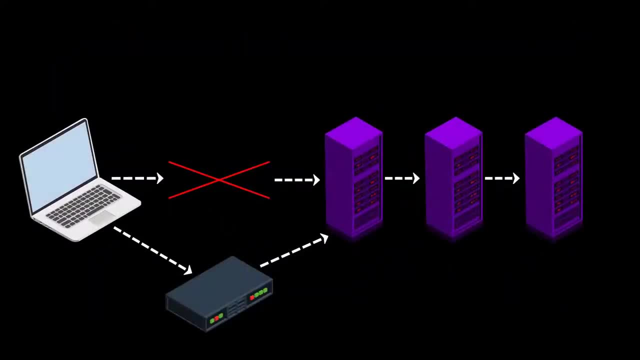 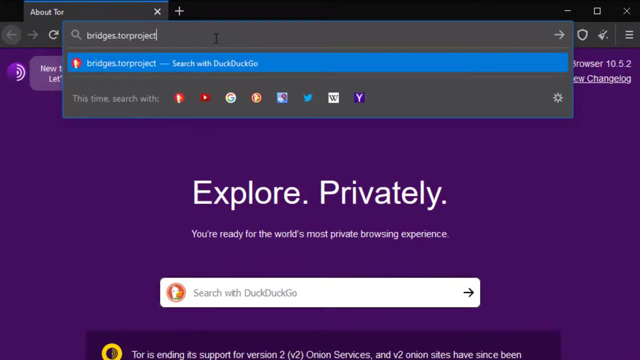 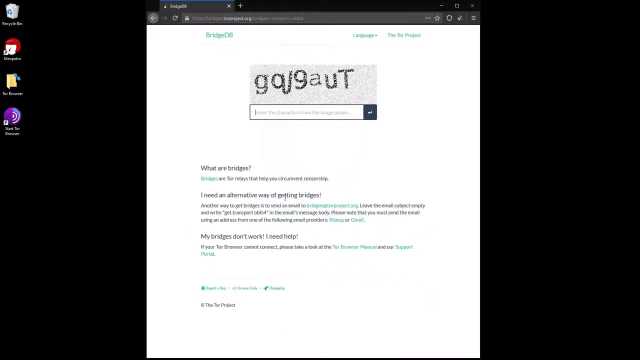 All bridge connections cannot be blocked at once. So even if the servers are blocked, access to the Tor network can be achieved over the bridge connections. So establish the bridge connection. you need to visit the bridgestorprojectorgoptions. After entering the security code, you can see address information required for bridge. 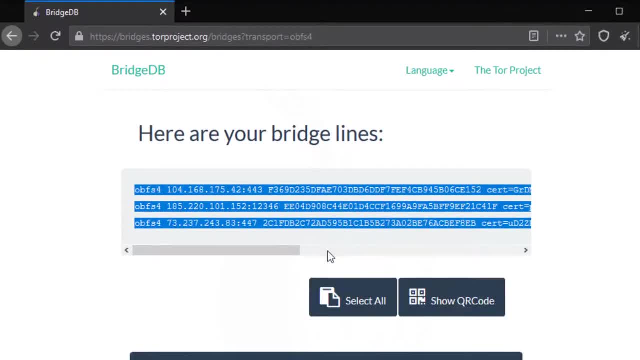 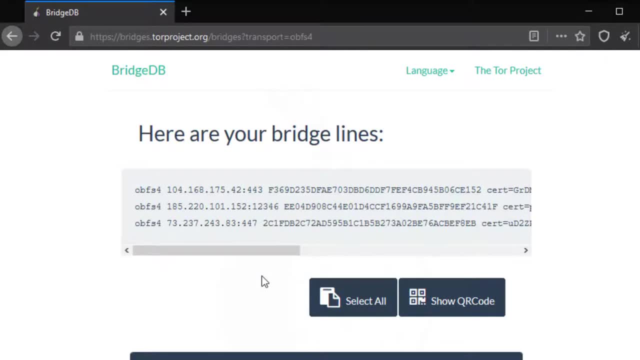 connections, You can copy these addresses from here. If Tor is blocked on the internet you are connected to, this website is probably also blocked. If you haven't been able to obtain bridge addresses in this way, you can access these websites using any VPN service. You can also get these addresses from within the. 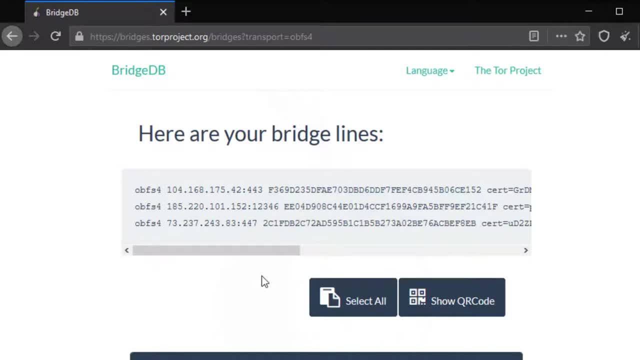 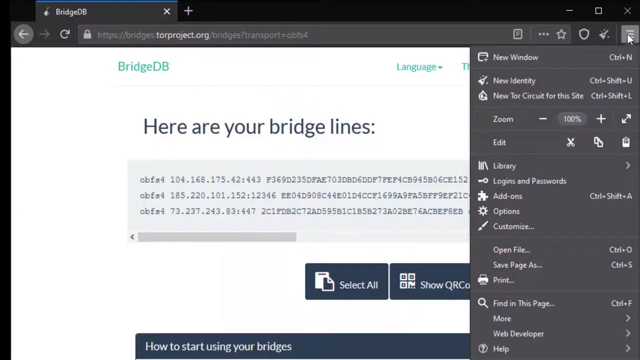 Tor browser as an alternative to the VPN option. When we talk about the Tor browser settings, you will see how it works. Now you can get bridge addresses from within the Tor browser. Now let's click the three line icon on the right side of the browser to open the menu. 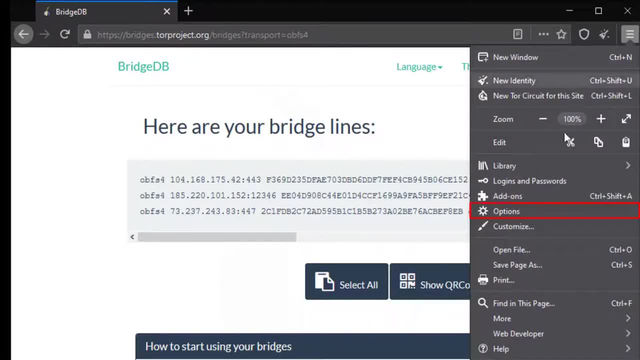 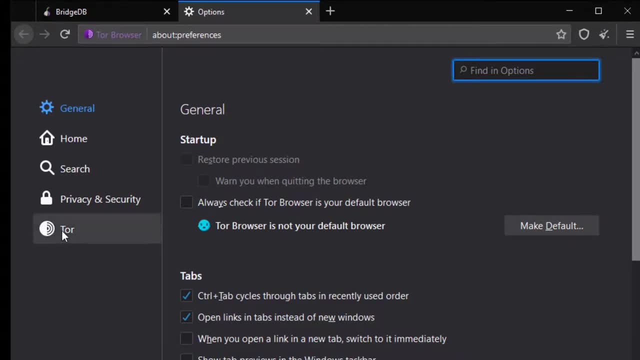 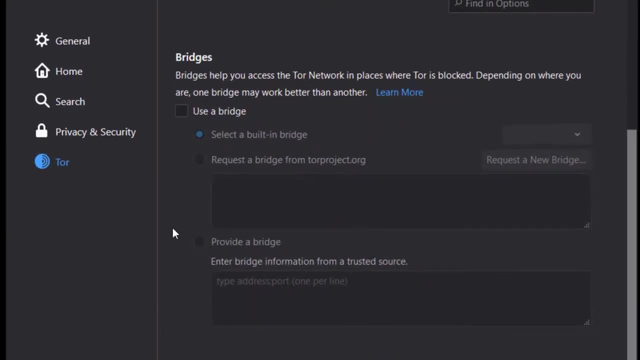 to make the necessary settings for the bridge, Click on options from the menu that's open. After the options window opens, click on the Tor tab on the left. Here we will make the necessary settings for the bridge connections. To configure the bridge. first let's checking. 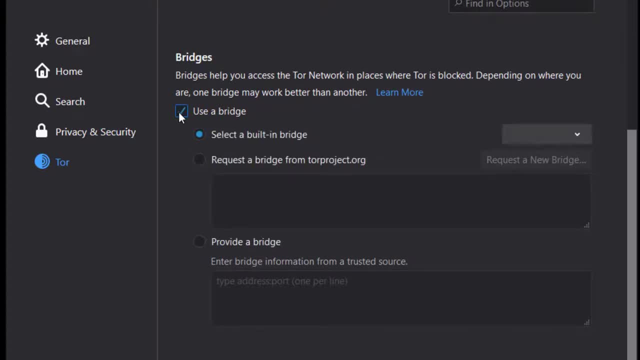 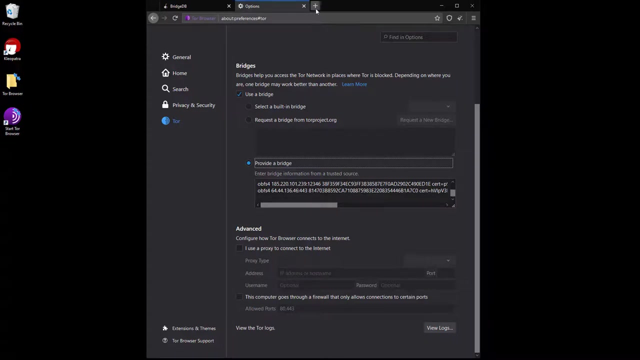 the use bridge box. If you have bridge addresses, you can click on the provide a bridge option and enter the bridge address in this field, Those the Tor network will be provided over the bridge connection you have specified. To test whether a bridge connection is available, let's go to checktorprojectorg again and 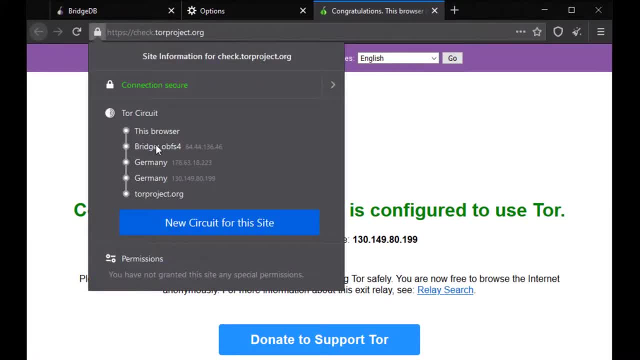 check the nodes used to connect to this address. As you can see, the first node is the bridge. This means that you were able to successfully establish the bridge connection. In addition, if you don't have addresses for the bridge connection, you can also use the. 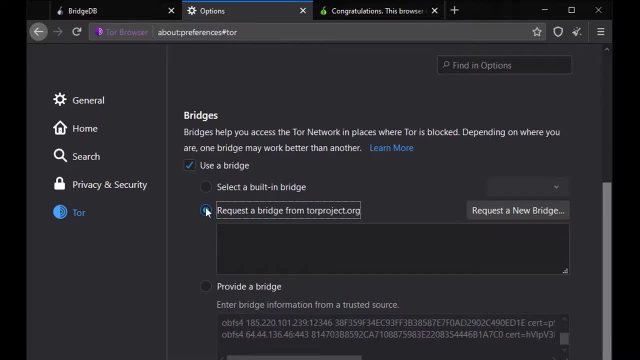 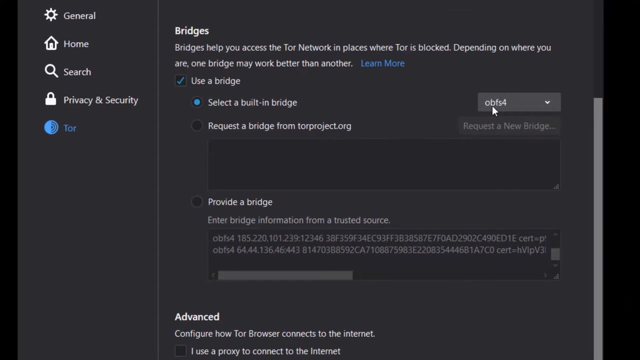 select a built-in bridge or request a bridge from torprojectorg options from the bridge section. If you use the select a built-in bridge option, select the OBFS 4 option here a built-in bridge will be used. In addition, the bridge addresses can be defined automatically with the request a new bridge. 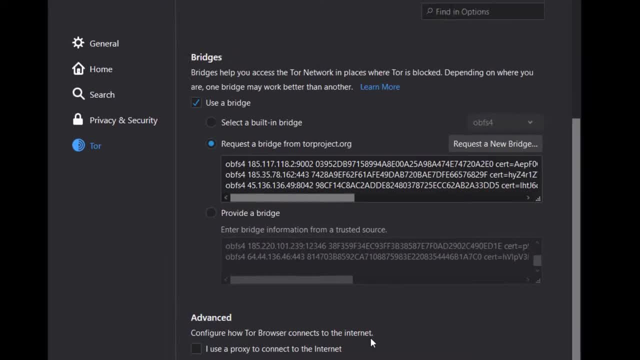 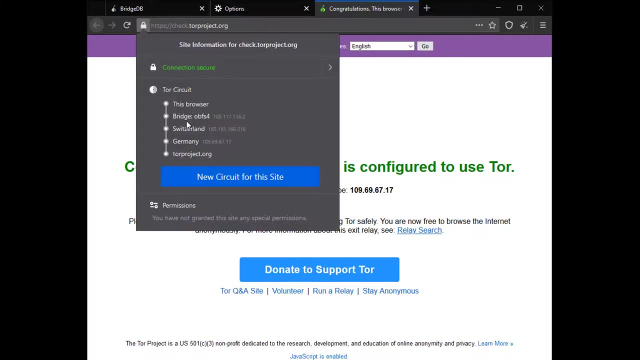 option. You can easily overcome situations where the Tor network is censored by using all these methods. If you are using the bridge connection and still have problems with the access, you are probably dealing with a censorship mechanism that detects that you have accessed the Tor. 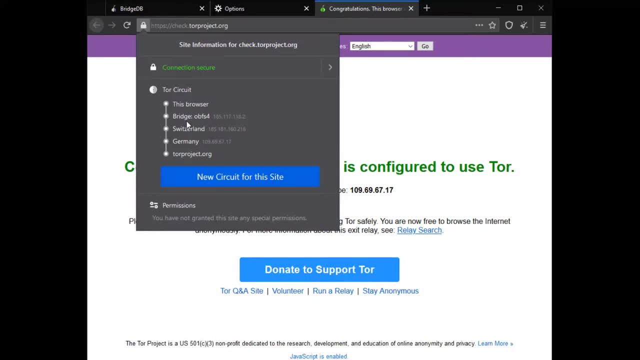 network by thoroughly analyzing your network traffic. As a simple solution to this situation, you may prefer to use the Tor network over VPN. However, using VPN will may provide you with much more security measures, as well as bypassing the censorship. If you don't have access block to the Tor network using a bridge connection won't make 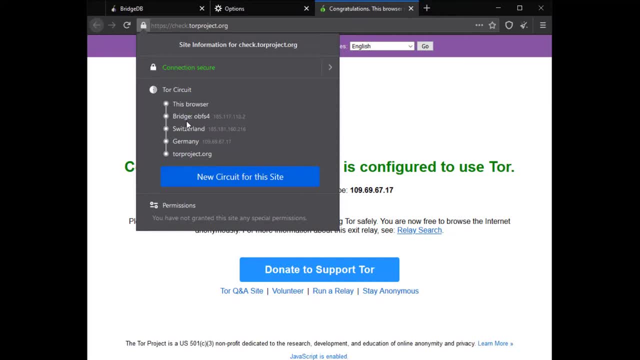 sense because won't provide you with extra security. Please note that the purpose of the bridge is only to bypass censorship, not to provide extra security. However, in some cases, you may want to use a VPN even if you don't have access block. 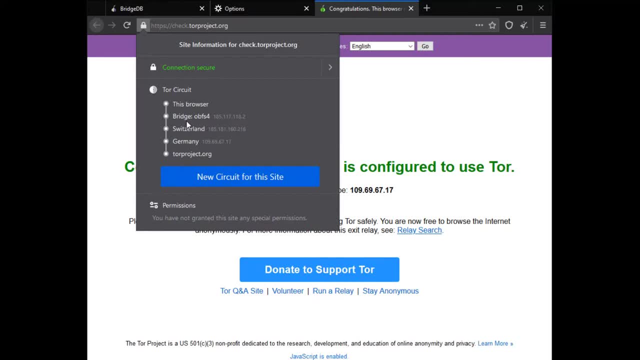 To better understand why, let's explain the effects of the VPN usage on the Tor network by handling Tor connection over VPN.